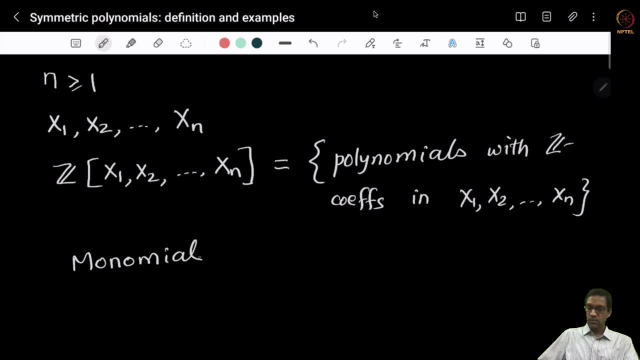 example of multivariable polynomial. It is what we would call a monomial. What is a monomial? It is just a single term of the following form: x1- raise to some power, x2 raise to some power, and so on. So xn. raise to some power, and monomial is therefore determined by the sequence of powers. 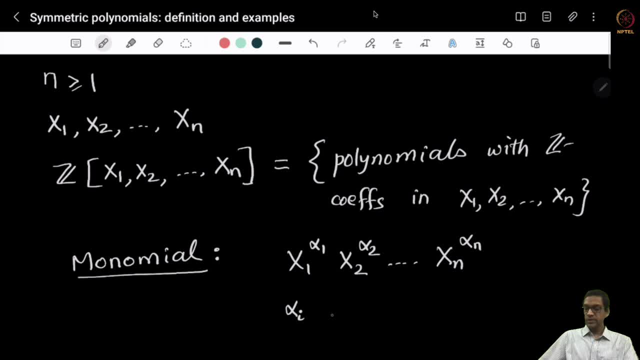 on top. So what are the alpha i's here, the powers? They are non-negative integers. So we use z plus to denote the set of all non-negative integers. These are all integers k, such that k is greater than or equal to 0. 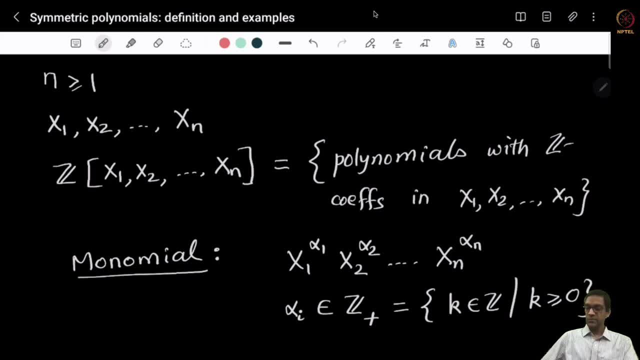 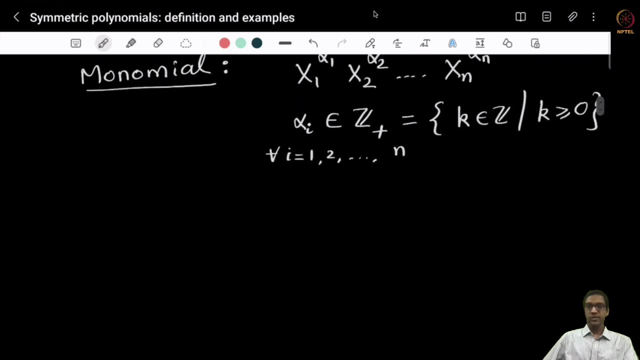 You can also call the alphais. these exponents belong to z plus for all i's. so I should say, for all i equals 1,2,3 till n. Now what we will do is we will encode this information as follows: so there it is: alpha. 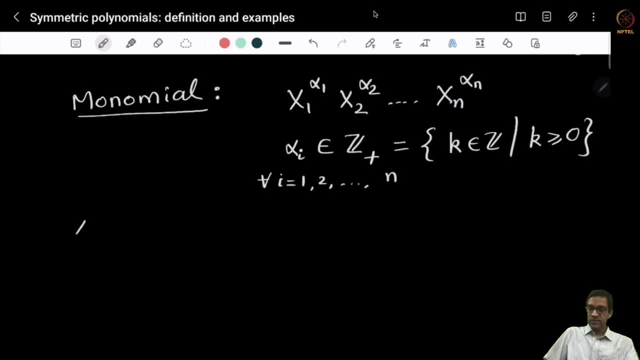 1,, alpha 2, and alpha n. It is well, it is actually a tuple. We should think of it as an육 order n en tuple: alpha 1,, alpha 2 and alpha n. So nowhere n n is indicated in dragged. 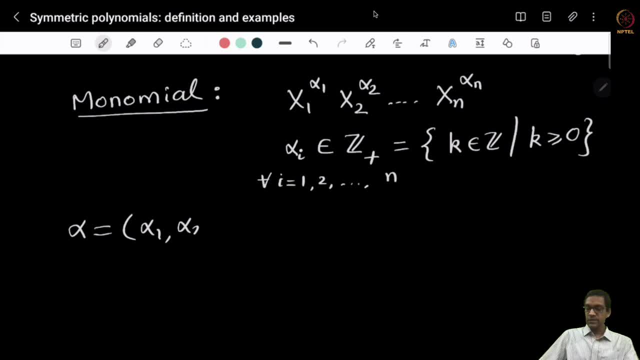 turn Now. of these, estos belong to z plus. for all is so, I should say for all. i equals 1,, 2, alpha n. this is an element of z plus power n, the Cartesian product of z plus, with itself n times. 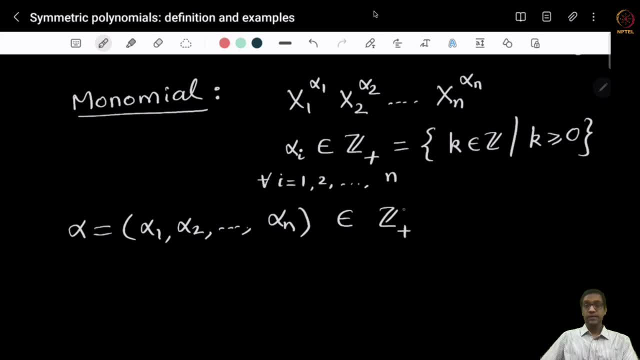 And this is sometimes called a multi index. So we usually call this a multi index. And here is some nice shorthand notation which is very, very convenient. We write x to the alpha for this monomial. So this is just notation, if you wish. Definition: x to the alpha just denotes: 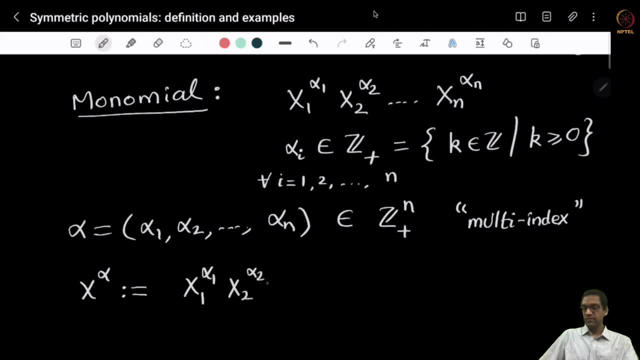 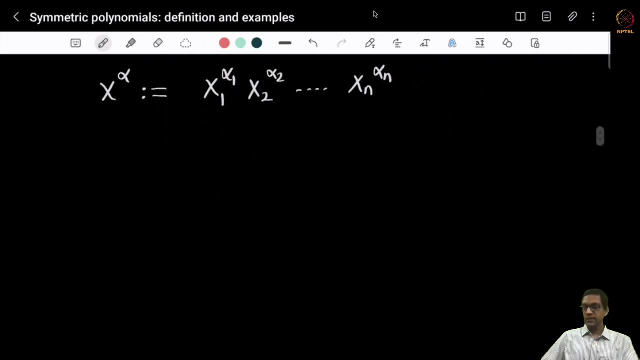 the monomial: x 1 to the alpha 1,, x 2 to the alpha 2, x n to the alpha 2.. Now observe that monomials are special for the following reason: that any polynomial is well, nothing but a sum of monomials. So observe the following simple fact, So fact, if you wish. 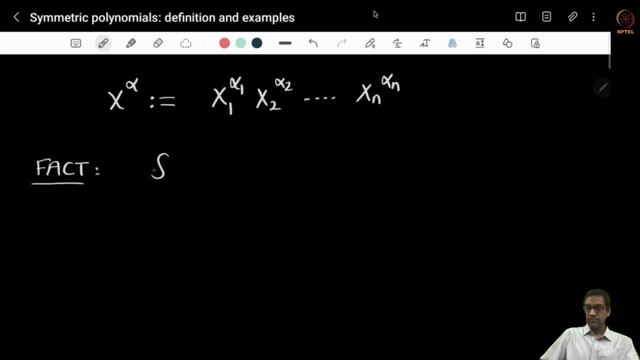 f is a polynomial, So f of x 1,, x 2, x n is a polynomial, So f of x 1, x 2, x n is a polynomial, So f of x 1,, x 2, x n is a polynomial. 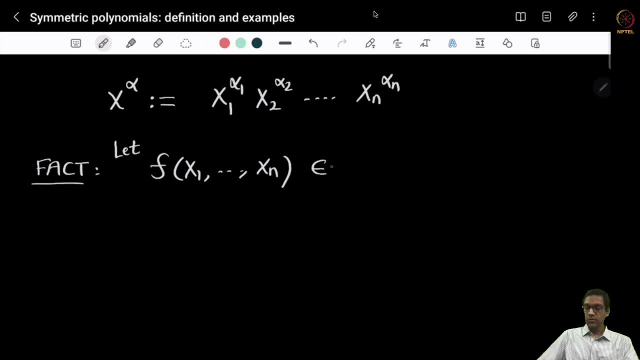 So let this be a polynomial in the n variables x 1,, x 2,, x n, Then f can be uniquely written as a linear combination of monomials. Then f of x 1,, x 2, x n can more or less by definition that is. 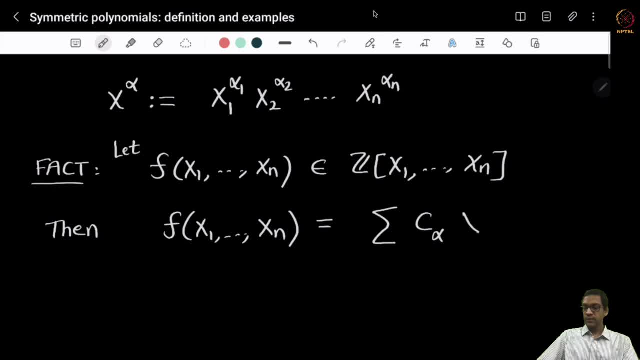 what a polynomial is can be written as follows: It is a linear combination, c alpha, x to the alpha, where alpha runs over the possible multi indices, z plus power n, and where c alphas are all integers and only finitely of them are not 0 and c alpha is 0, except for finitely many multi indices alpha, except for: 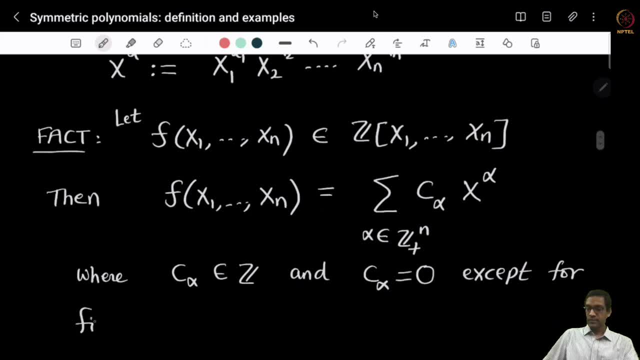 finitely many And further. this expression is unique. that is the other, more or less obvious fact. So this is why monomials are important. They are most natural basis, if you wish, in terms of which a polynomial can be expanded. Here is a simple example. So 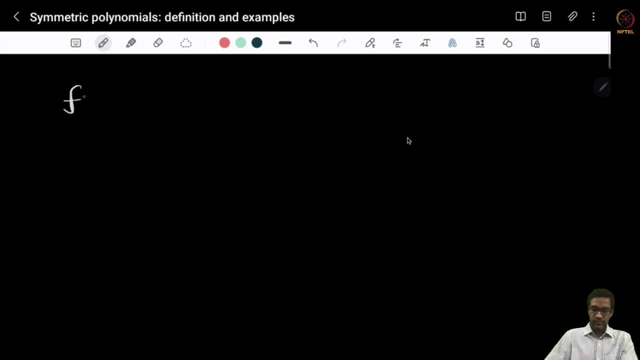 we could take the polynomial f of x to be x 1 cubed, x 2 square, x 3 power 1 plus x 1 power 1 x 3 square. Now notice I use just the variable letter x here, So x here already is a shorthand. 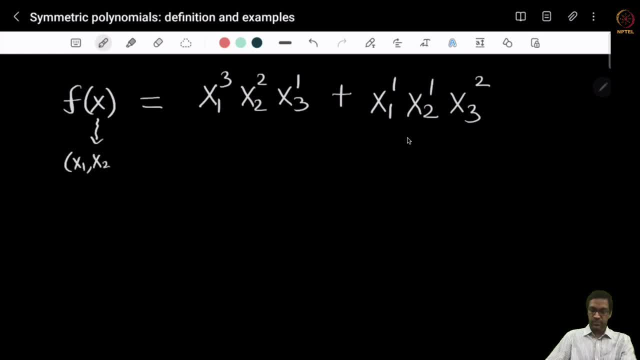 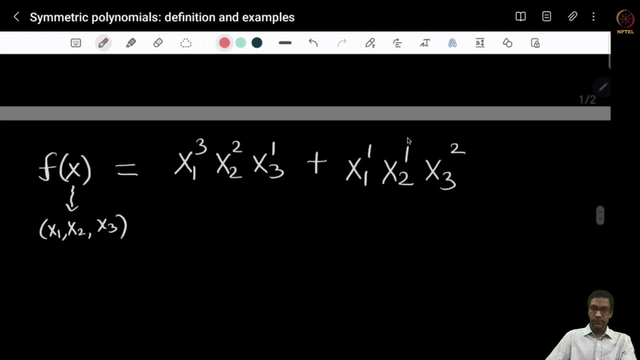 for the tuple x 1,, x 2,, x 3.. Now so here is a polynomial which is the sum of two monomials, and what are the multi indices here corresponding to the first term, For example, is so: 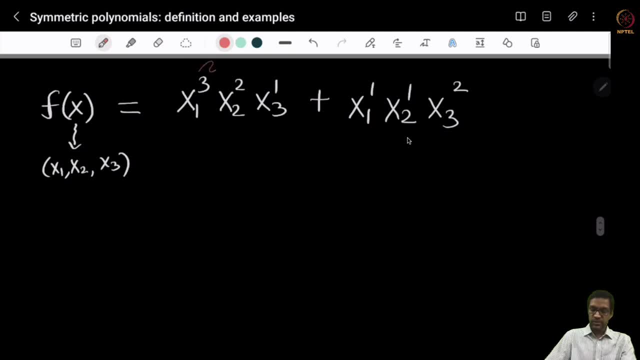 if you look at the powers which appear. so I got the powers 3, 2 and 1.. So they form the multi index 1 and for the second term the powers are 1, 1 and 2 and so the multi index corresponding. 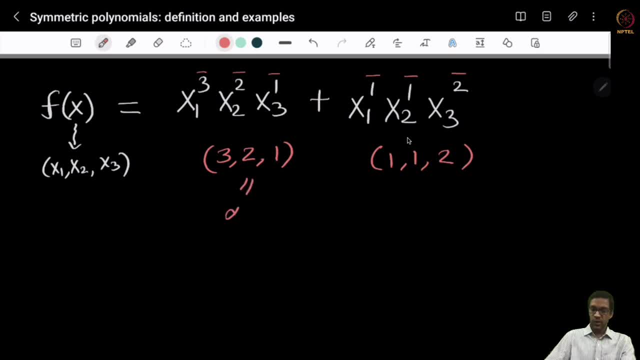 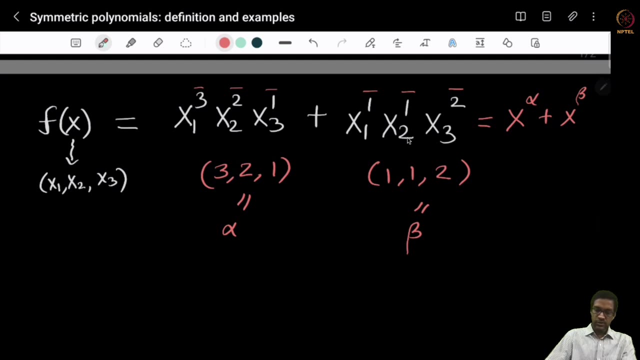 to that term is 1, 1, 2.. So in other words, if you call this as alpha and this as beta, then the given polynomial is nothing but the sum of the monomials in our notation: x to the alpha plus x to the beta. So this is sort of useful shorthand, because when we start 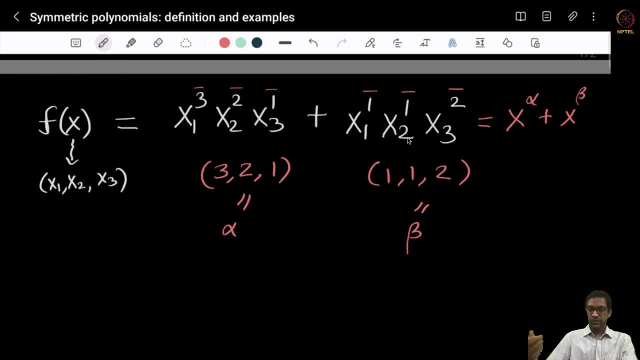 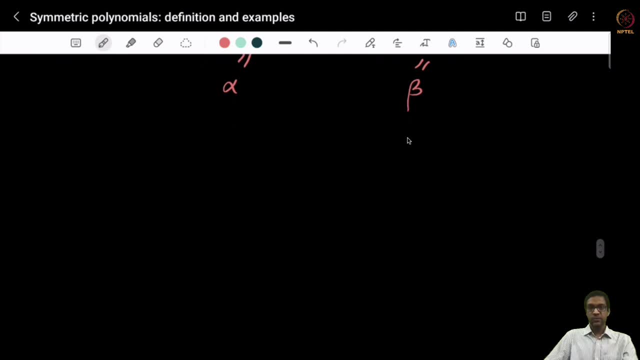 talking about symmetric polynomials. we will need to. you know, we will be dealing with many, many terms and the indices are somehow the exponents. the multi indices will be the easiest way of describing various properties. ok, So now to the main agenda of this lecture, which 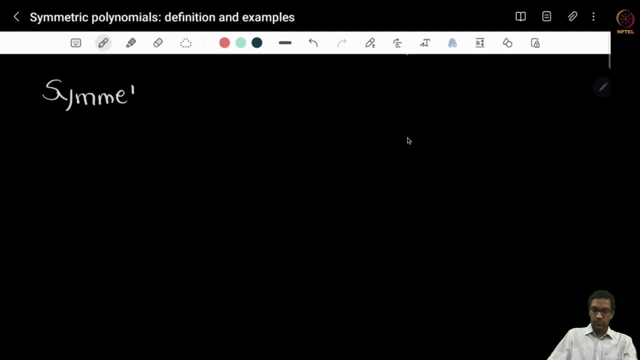 is to talk about what symmetric polynomials are. So what do you mean by a symmetric polynomial in n variables? So a polynomial f is said to be symmetric, So this is a polynomial in the variables. let us say So, this is in x 1, x 2, x n. 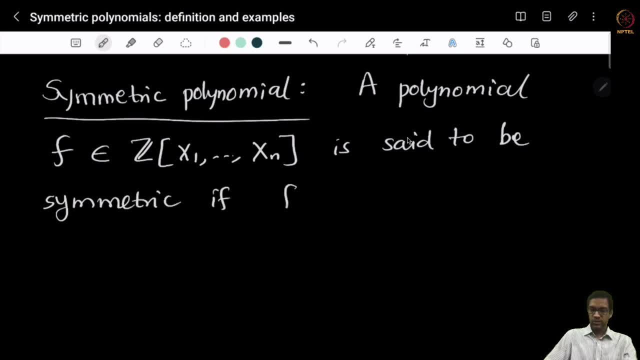 Symmetric. if The following holds: f of x 1, x 2, x n, polynomial is the same as f of any permutation of the variables. ok, So if I change the order of the variables in any way I want, So let us. 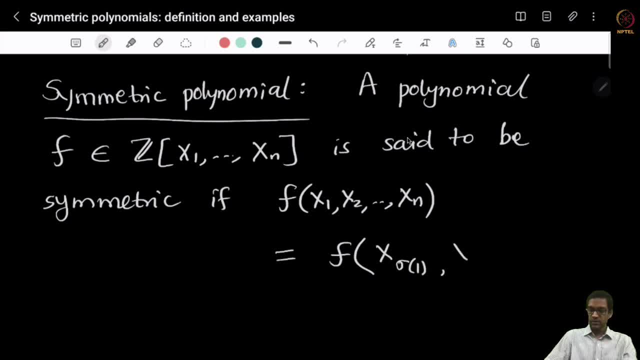 describe it as follows: I permute, So I look at, instead of x 1, x 2, x n, I look at x sigma 1, x sigma 2, x sigma 3, x sigma 4, x sigma 5, x sigma 6, x sigma 7, x sigma 8, x sigma. 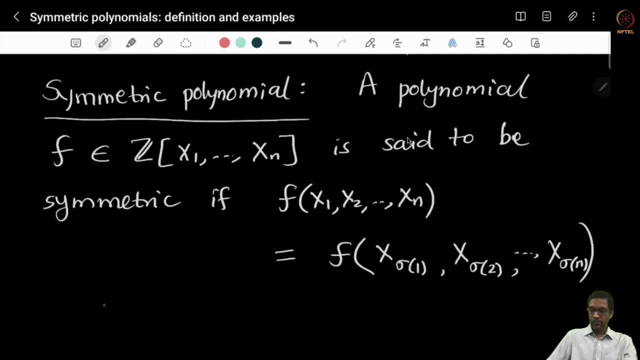 9, x sigma 9, x sigma 10, x sigma 11, x sigma 12, x sigma 13,, x sigma 14, x sigma 14, x sigma 15, x sigma 12, x sigma 15.. 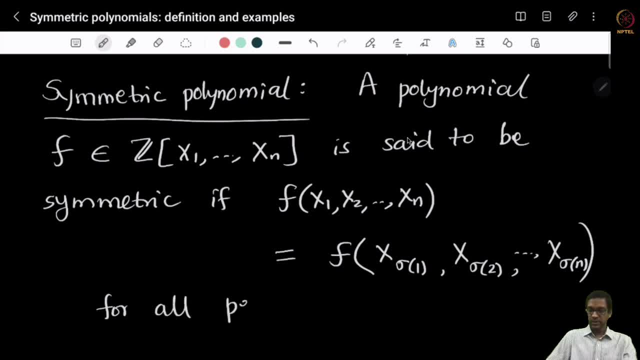 For all permutations sigma. So this should be true for all permutations sigma of the numbers 1 to n. ok, So recall the usual terminology here: the group, the permutation group s n is nothing but the set of all permutations of n distinct symbols. So here I am going. 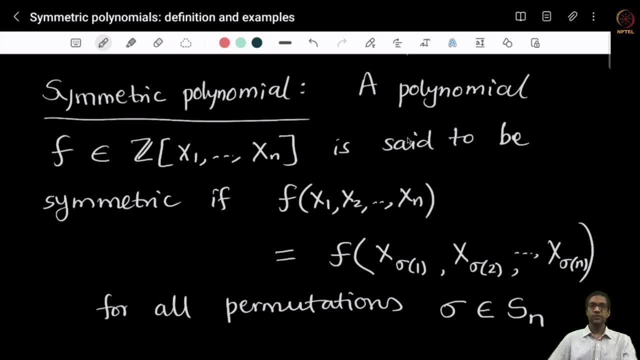 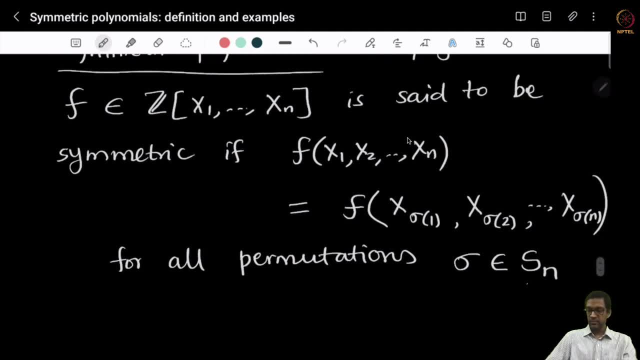 to think of S? n as being the set of permutations of the numbers 1,, 2, 3 till n. So this Sn is exactly the set of permutations of the numbers 1 to n. So any which way you permute the variables, the polynomial f remains the same. 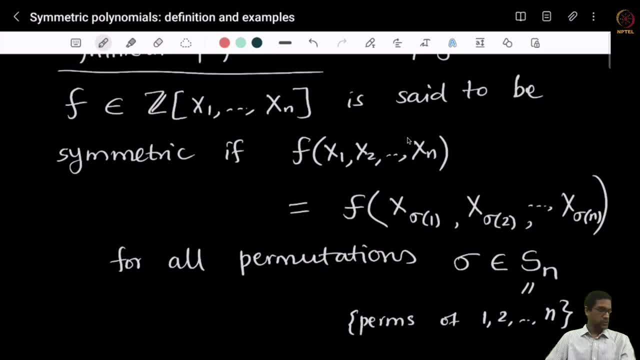 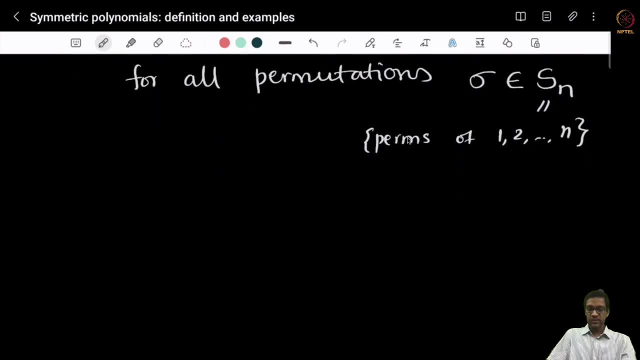 So that is the definition of a symmetric polynomial. So what are examples? So let us look at simple ways in which one can construct symmetric polynomials. So let us start with n equals 2.. So two variables. So what is the property here? 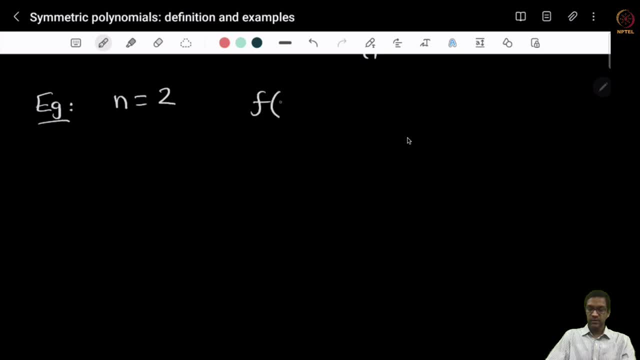 So I have two variables, x1 and x2, and the property that I need to satisfy really is only this: that if I permute the variables like this: look at x2, x1, then the value of f is the same. So this is what a symmetric 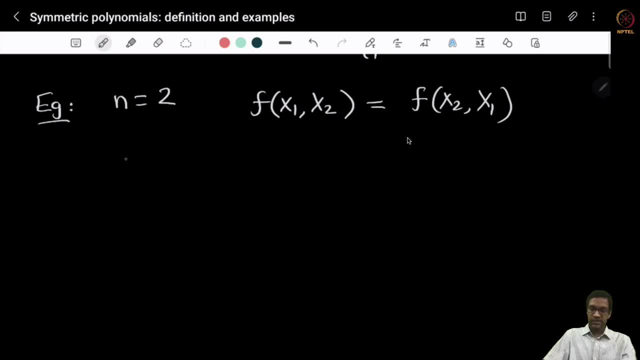 polynomial is. So this is symmetric polynomial. So let us write an example. Let us write a few different examples, So I could take, for example, f of x1, comma x2 to be, for example, just the sum x1 plus x2.. Here is an example of a symmetric 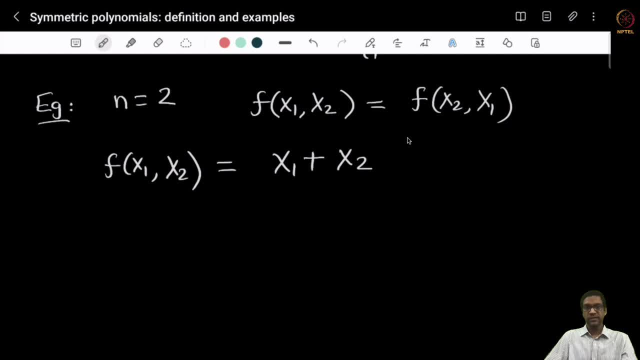 polynomial. If I change the variables x2, x1, I just get x2 plus x1, which is the same thing. So this is one example. Example 2, I could look at the polynomial f of x1, x2 equals. So this is polynomial 1.. Here is 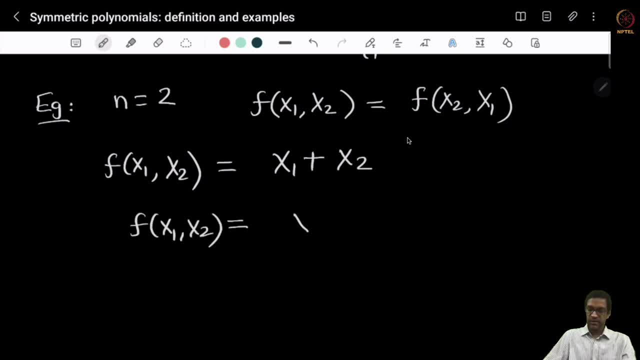 the second f of x1, x2 equals. for example, let us say I want the monomial x1 square x2 to be part of my polynomial. Now the only way this resulting polynomial can be symmetric is if I also add in the sort of symmetrization of this, meaning I change x1 to x2 and x2 to x1.. 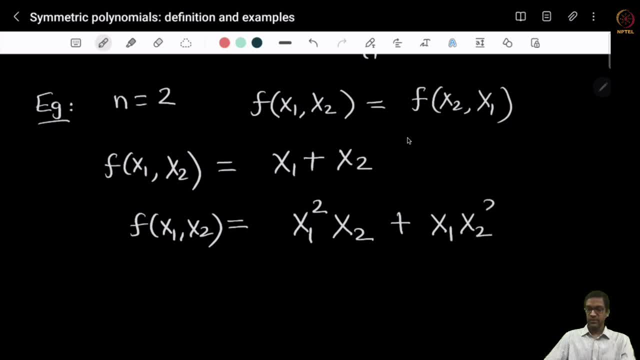 So that will become x1, x2 square. So observe now I have done the least possible to make it symmetric. This is an example of a symmetric polynomial: two variables. Let us take another one, So just like the very first one, or maybe let us take something slightly more complicated, So for 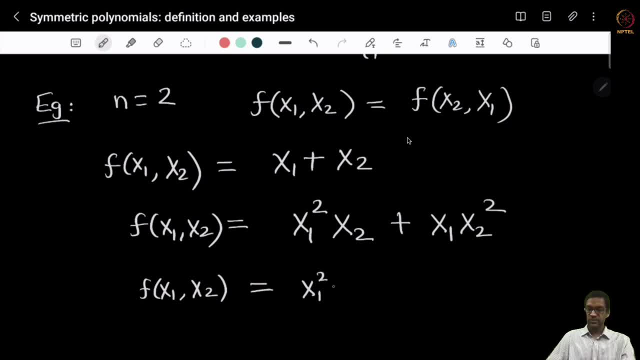 example, I can take x1 square plus x2 square, which is like the first example, except I have not squared both variables. But let me now also do the following. So observe: this is by itself already symmetric, but I could also add something further to it. So let me do the following. 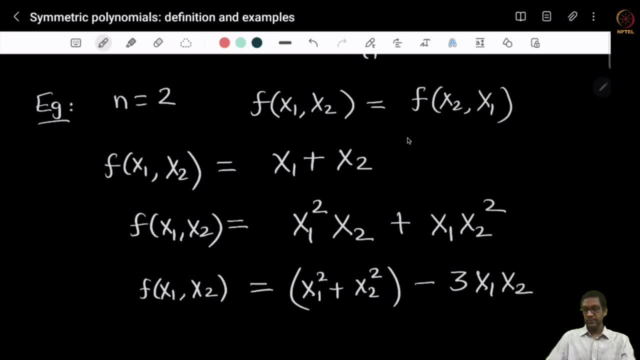 I say this minus 3 x1 x2.. So observe that this resulting thing is symmetric. also, Why? because the first term, x1 square plus x2 square, is symmetric under interchange of variables. and so is the second. So this is symmetric because the first term, x1 square plus x2 square, is symmetric. 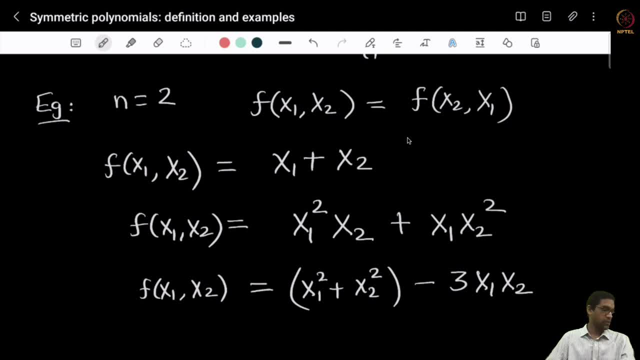 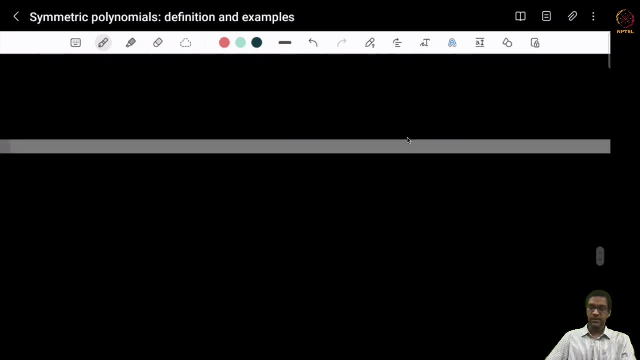 term. So here are some examples of symmetric polynomials. Now of course you can imagine that as the number of variables increases, you can sort of construct far more complicated examples. So let me just do one for n equals 3.. If I take the polynomial f of x1,, x2, x3,, 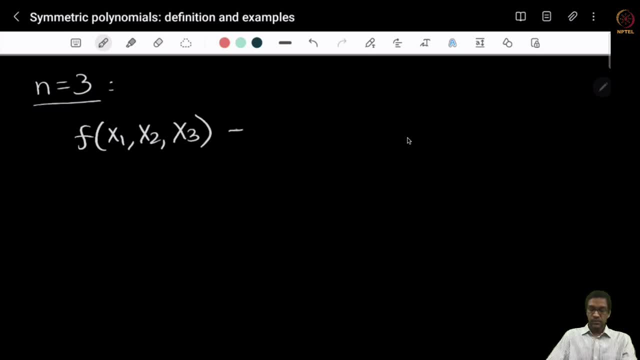 let me say I want the following: I want x1 cubed, x2 squared, x3 power1.. I want this monomial to be part of my polynomial f, but I also want it to be symmetric. So what is the least I should do? I need to add in some extra terms, which are obtained by sort of. 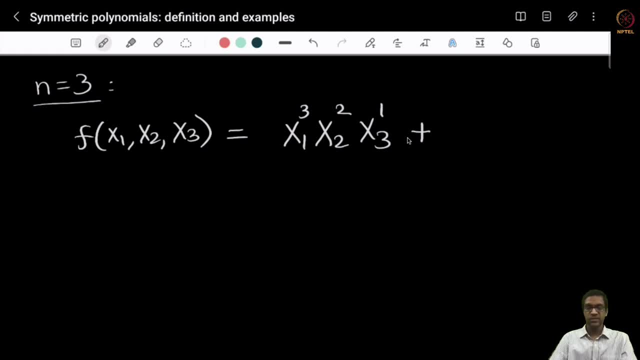 symmetrizing, permuting the variable, In other words قرب ξ of x1 will be función withclip 갯 gak andTherefore shadethe sum of the property be одну μ failure and then cac of τ will give you sm each zero and 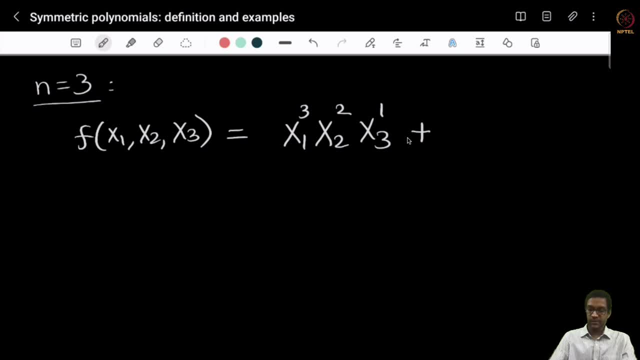 stands. this is not symmetric, but let me make it symmetric. well, what will i do? i will, for example, look at permutation. so let me first interchange x1 and x2. okay, so i will get, instead of x1 cube, x2 square, i have x2 cube, x1 square, x3. okay, you can of course rewrite it as x1 square, x2 cubed, x3. 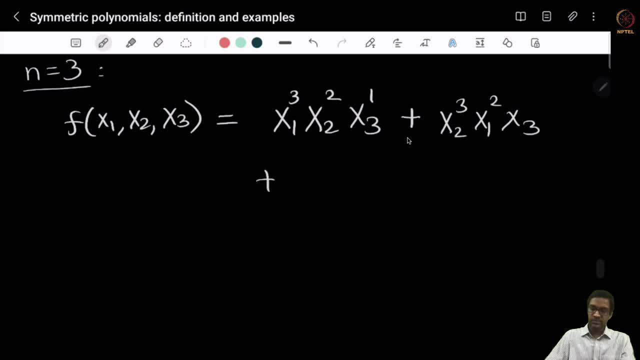 okay, and plus, what else can i do? how else can i interchange my variables? uh, so i left three in three constants, so now i will keep one in its place i, and i interchange the other two variables: x3 square, x2 power, one, okay. or i leave two in its place, x2 square, and i interchange one and three. 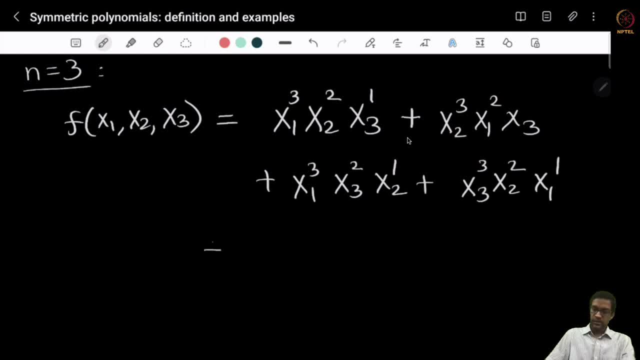 okay, so three to one. okay, so i've done three of the permutations, but there are some more. there is these, there are these cyclic permutations, for examples. okay, so, um, what are my other permutations? uh, i have cyclically shift the three variables. so one goes to two, two becomes three, three becomes one, and the powers are still three to one. then there's the. 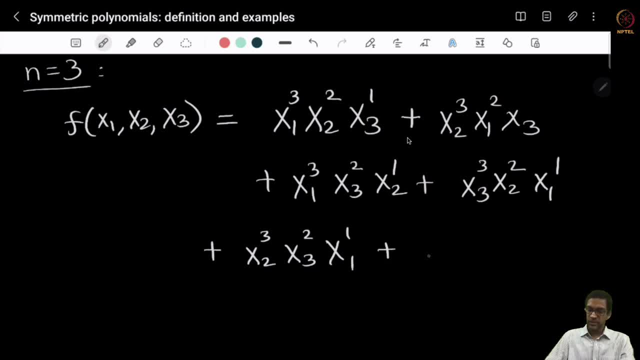 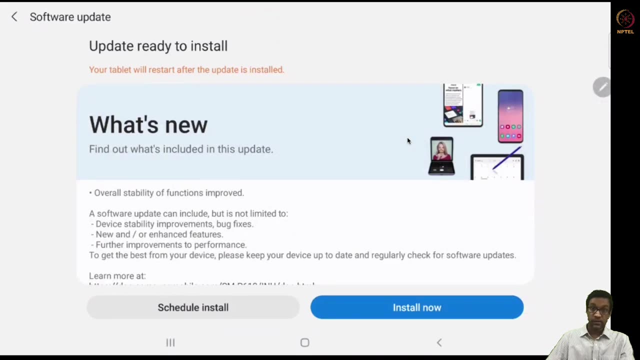 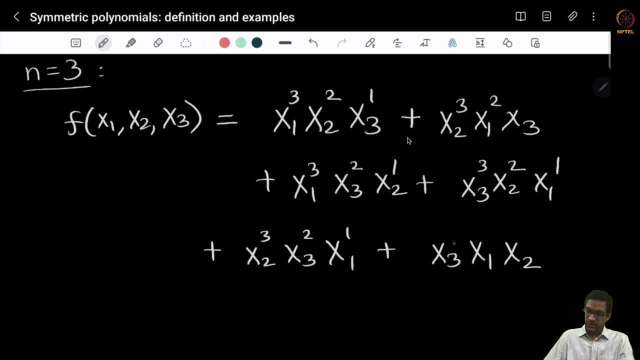 other reverse cyclic shift, which is: uh one becomes three, uh, two becomes one, three becomes two. okay, so two, three, one is one of them, and then three, two, one is another one. okay, so three, two, one. uh, three, one, two is another one. so this will now become uh again. cubed square. 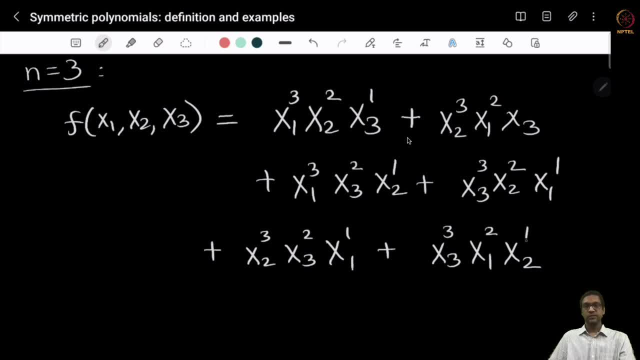 one. okay, so that's uh. so what have i done? i've sort of written out six terms and now you can check that this resulting polynomial- this is the sum of six polynomials- is actually a symmetric. okay, why? because any, any permutation of the variables i i take. 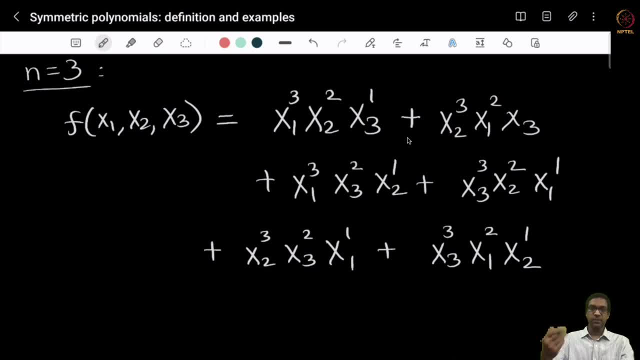 i will. i'll get back the same polynomial, i will get the same six terms, maybe in some other order, if i permute the variables. but it's not just that. i can, of course, do more complicated things, like i did earlier. i can say: okay, i take four times all of this plus, let's say, some other constant. 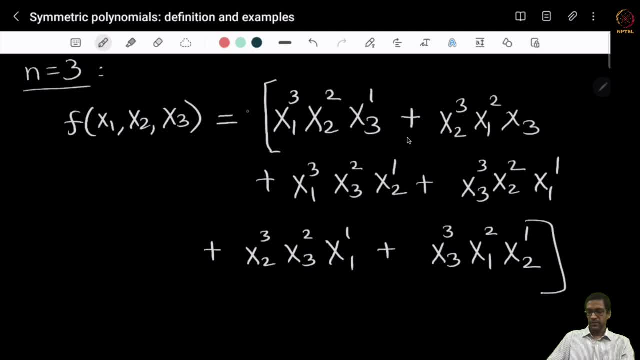 three times, maybe x one, uh plus x two plus x three. okay, this is also symmetric, okay, so all i've done is just uh, added to it an additional term and ensured that that additional term is also symmetric, okay. so here are some complicated examples. maybe, and- and as you can imagine, you can manufacture uh still more complicated examples as you. 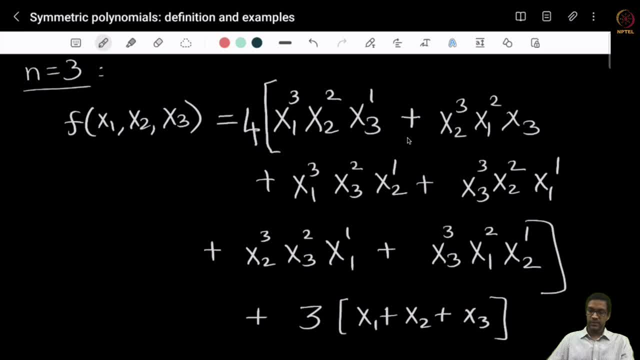 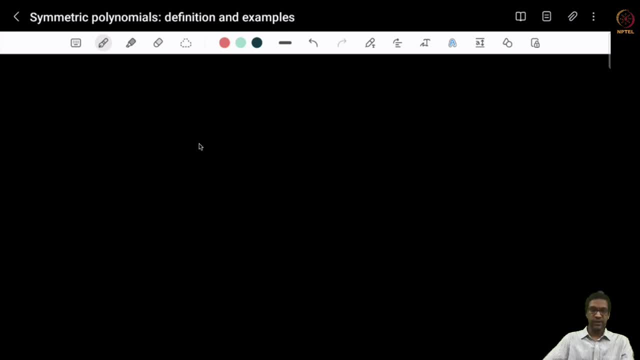 increase the number of variables, okay, good, so let's, uh, let's try and record the basic observation that we have made so far while we try to construct these examples, so something that that we actually have observed already. so here's the proposition. it says that, uh, okay, let's. let's start with the 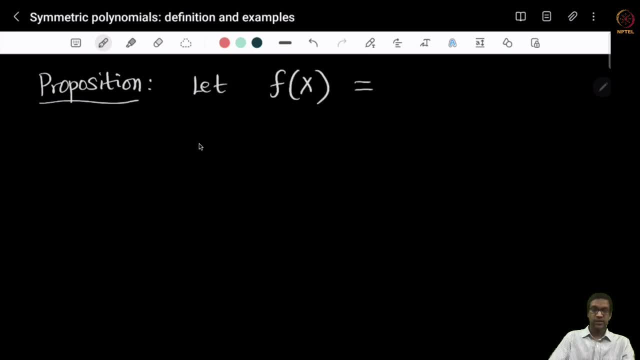 polynomial. let f of x. so x, here again is a, is a multi-index. you know many variables: x, 1, x, 2, x, n. so let f of x, uh be a, be a polynomial. so let me call it summation c, alpha x to the alpha. so recall. any polynomial can be written like this: 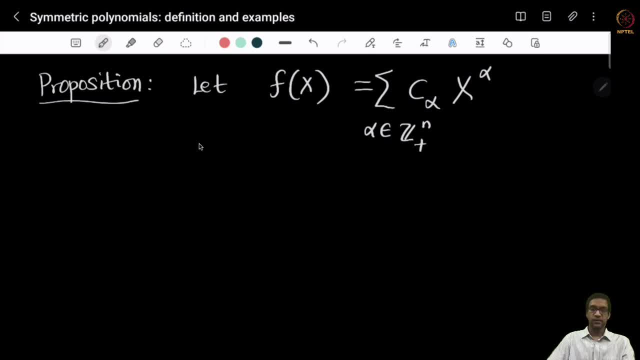 here with finitely many terms, and c alpha is being non-negative integers, so as described before. so let this be a polynomial in n variables, then the symmetry of f, then f is symmetric, f is a symmetric polynomial. so the point is that f of y is the same as saying that it says something about the, the coefficient. 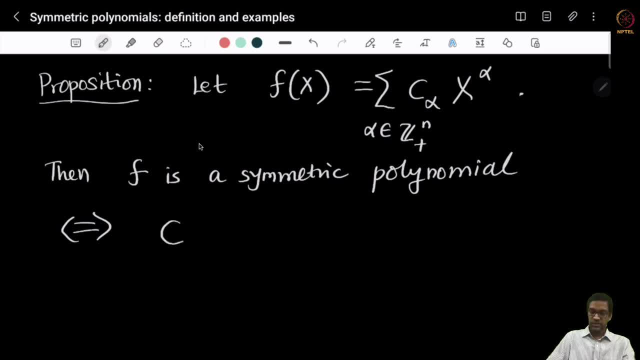 c alpha. it says that the coefficient c alpha, that is, the coefficient of the term x power alpha, is the same as the coefficient of the term x power beta, where beta is some permutation of alpha. okay, so that's. that's exactly what we have observed when we constructed these. so 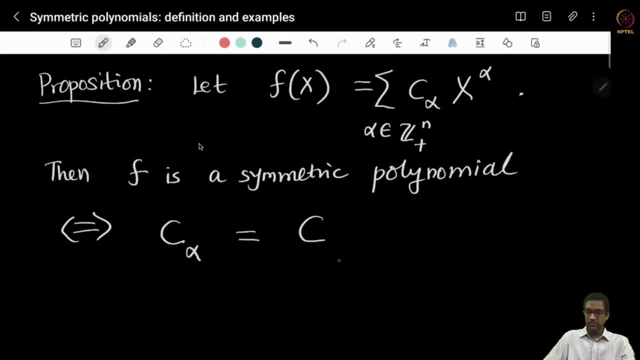 alpha is the same as c. well, how shall we write this? so let us, let us do the following. let me write alpha out in full, so I will call this: c of the multi-index: alpha 1, alpha 2, alpha n, that is the coefficient of the monomial x1 power alpha 1, x2 power, alpha 2, and so on till xn power. 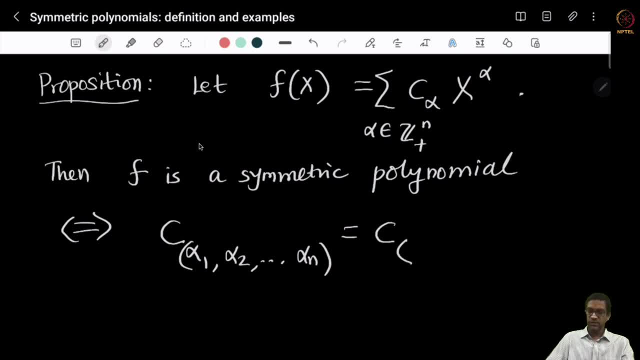 alpha n. this is the same as the coefficient of the monomial. where in place of alpha 1, I have some other alpha i, I have some other, some permutation of these n guys. so let let me call that permutation something. so instead of alpha 1, I have alpha tau 1, instead of alpha 2, I take. 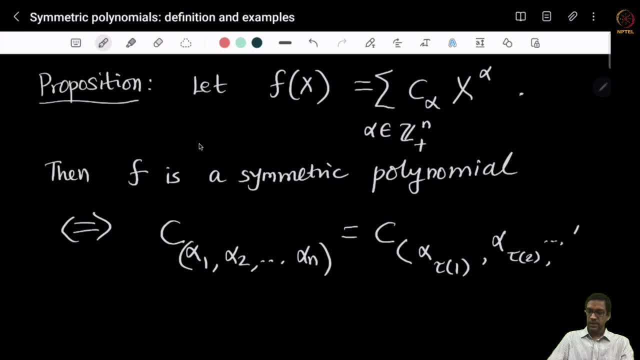 some other guy: alpha tau 2 and so on. alpha tau n, where tau is some permutation of the numbers 1 through n. okay, this should be true for all permutations, for all tau in a sen and for all alphas and all. so all the multi indices which are clear, okay, so observe, of course, most of the multi indices, most. 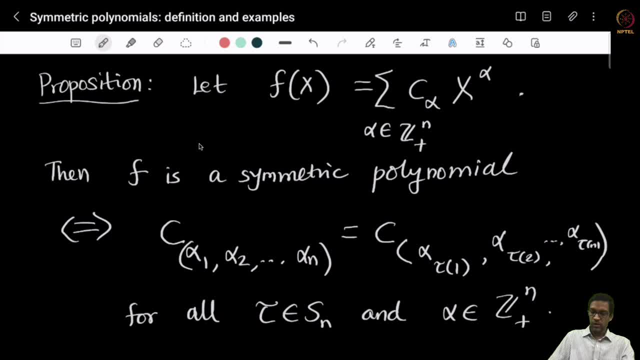 of the coefficients are going to be 0, right? remember, only finitely many coefficients are non-zero. so this is really a statement about those finitely many non-zero coefficients. that, if you know, if some coefficient of some monomial is is a certain number, then 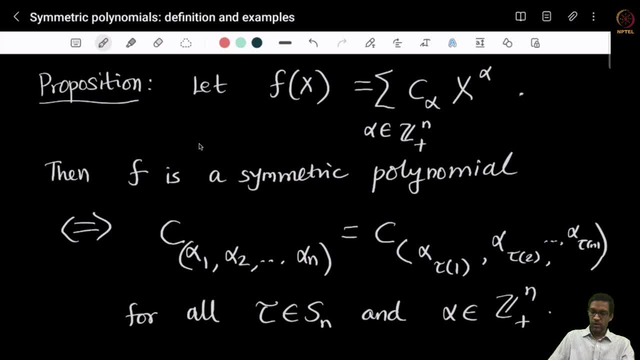 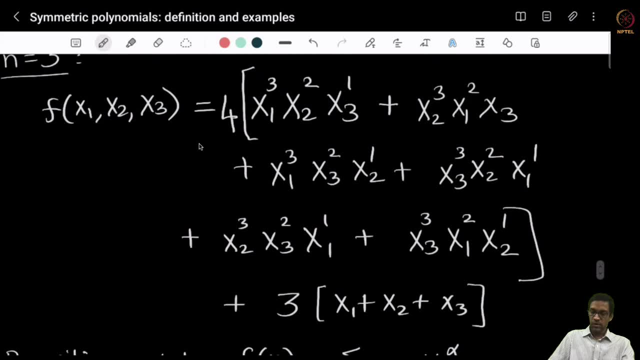 the coefficient of the permuted monomial should also be the same. okay, and observe, we already saw this in this, in this earlier example. so what did we have, you know, if you looked at all these monomials here? so this, this, this and so on, these six monomials. 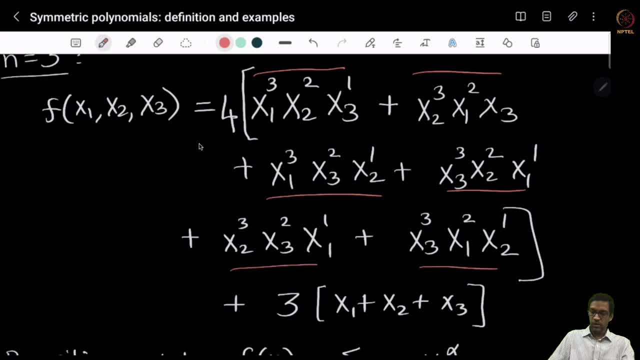 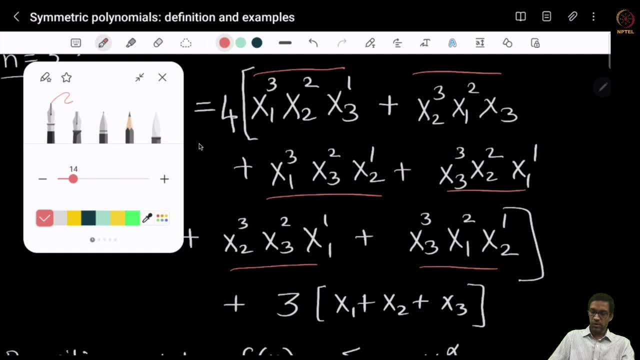 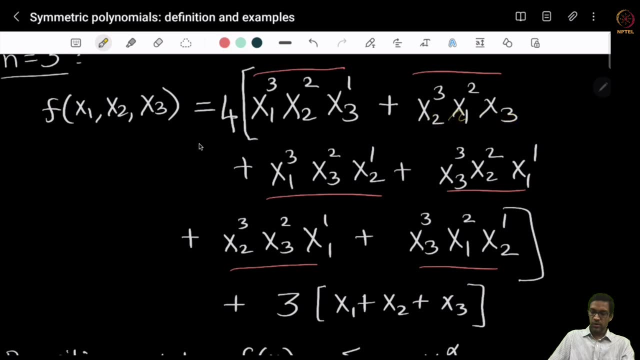 which correspond to permuting. think of it as permuting the alphas. okay, so why is it a permutation of the alphas? so if you, if you look at this, see this, this guy here, x2, cubed, x1, square, x3 is actually. so you can rewrite this, this term, as follows: so let me just rewrite this, this particular. 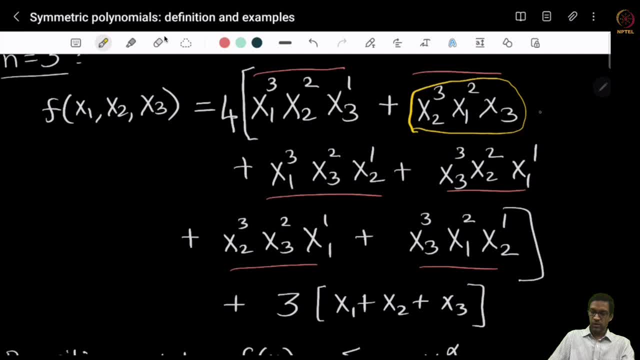 term here. this term is the same, as i will read it in the correct order: x1, followed by x2, forward by x3. then i can think of it as two, three, one. okay, in other words, i can either think of it as: so this particular term is equal to this, so i can either permute the variables or, equivalently, i'm. 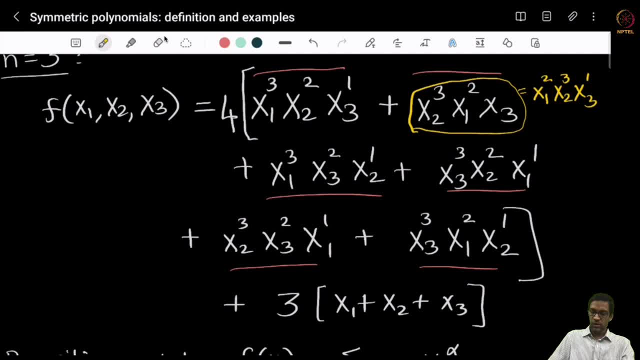 think of the variables as being fixed in their places, but the exponents are being permuted. So observe: instead of 3,, 2, 1 being the exponents, this guy has 2,, 3, 1 as the exponents. 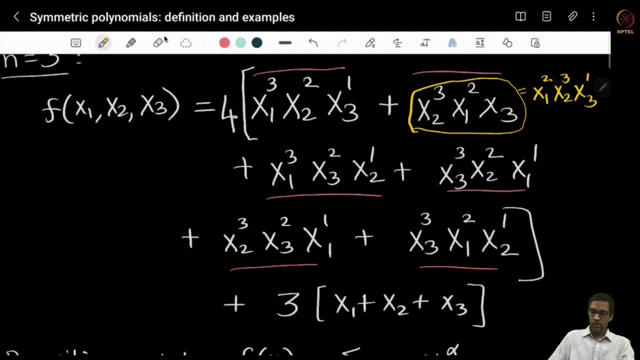 but now the x1,, x2, x3 are written in the correct order. So that is really what is going on here, that all these 6 monomials can be thought of as follows: you fix x1, x2, x3 and you permute the 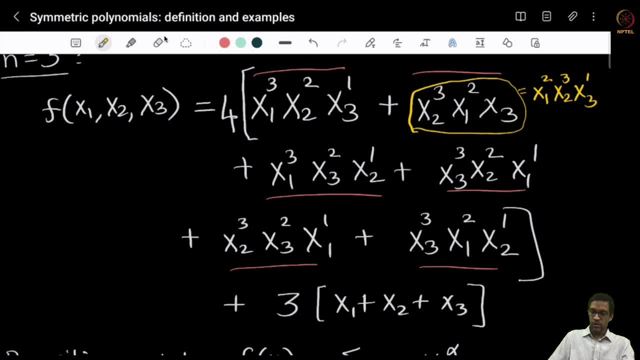 alphas and all permutations of the alphas, those different monomials that you get. all of them have the same coefficient: 4.. Similarly, likewise this monomial here: x1, x2 and x3. well, what do they correspond to? you should think of it as this is: x1 power 1, x2 power 0, x3 power 0. So it is the. 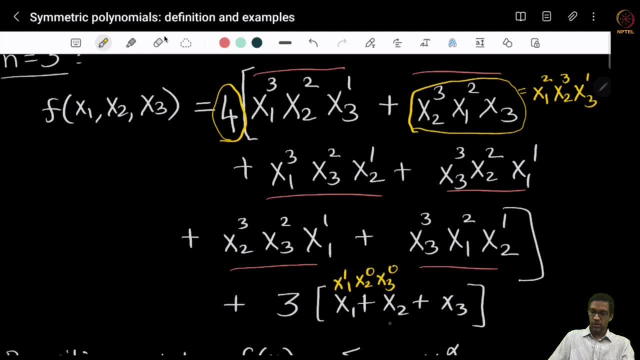 multi-index alpha is 1, 0, 0 in this case And for the second term, alpha for x2. what is it? It is 0, 1, 0 is just x1 power 0, x2 power 1, x3 power 0 and this third. 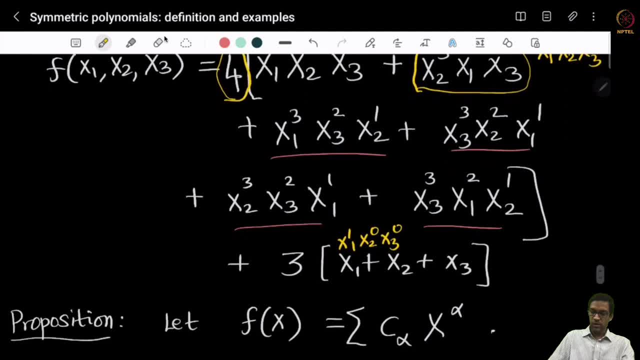 guy, x3 is just x1 power 0, x3 power 1.. So 1, 0, 0, 0, 1, 0 and 0, 0, 1, those are those 3 terms and 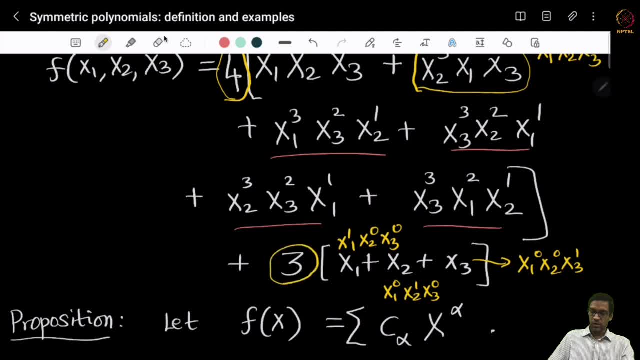 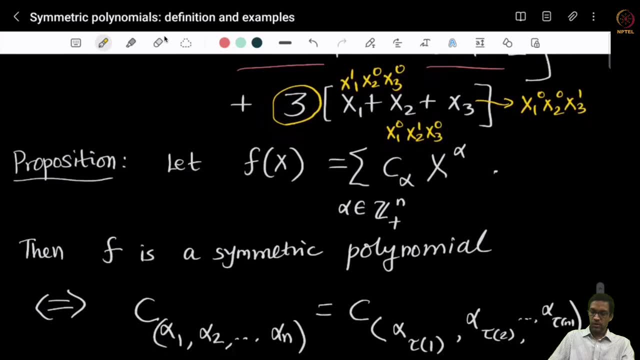 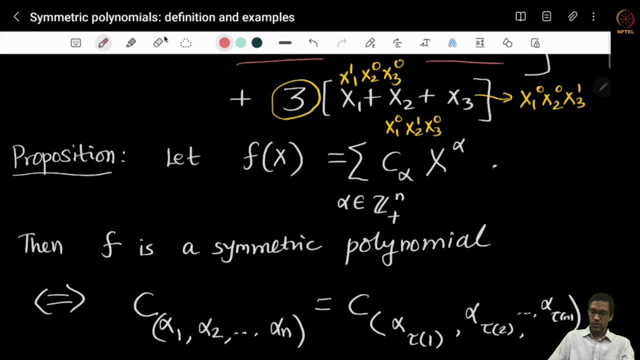 all of them have the same coefficient, namely a, 3.. So that is really what this proposition is: saying that if you write f- So here is the proposition- if you write f of x as a linear combination of monomials, then f is symmetric. is the same as saying that the 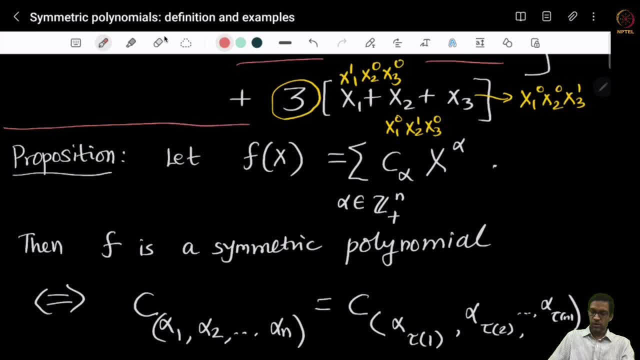 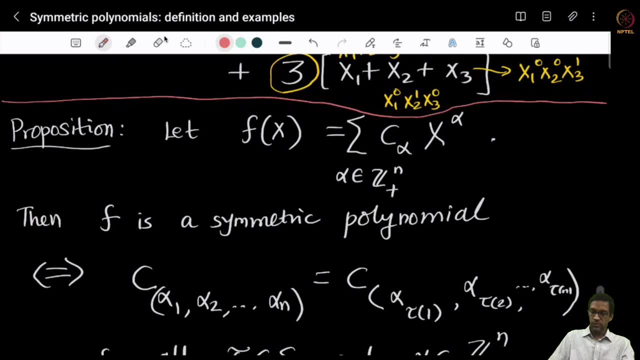 coefficients c alpha will turn out to be the same as the coefficient of the monomial you know, which is a permutation of alpha. So that is the first proposition. the proof is more or less obvious from what we have said before. but let us do it now. plus at least I will indicate. 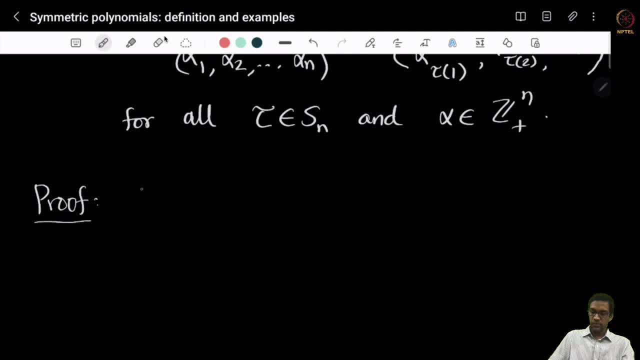 how to formally write this out. So let us prove the forward direction, which is: if f is symmetric, then this particular property holds the coefficient equalities. So observe: f is symmetric says the following: So f is given to be symmetric. So f is symmetric means what? So the defining property of symmetry says: 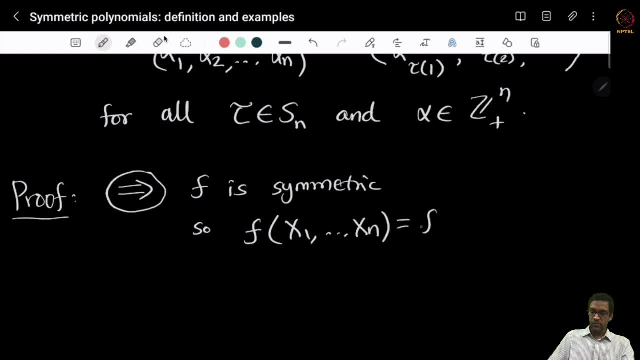 I can permute my variables and the polynomial will not change. So let me take that same permutation. I will pick a permutation, tau. So I will look at x tau 1, x tau 2, x tau n. this is true for all tau permutations, of 1 to n In particular. now what? is that mean I will expand the polynomial? So I will look at x tau 1, x tau 2, x tau n. this is true for all tau permutations of 1 to n In particular. now, what does that mean? I will expand the. 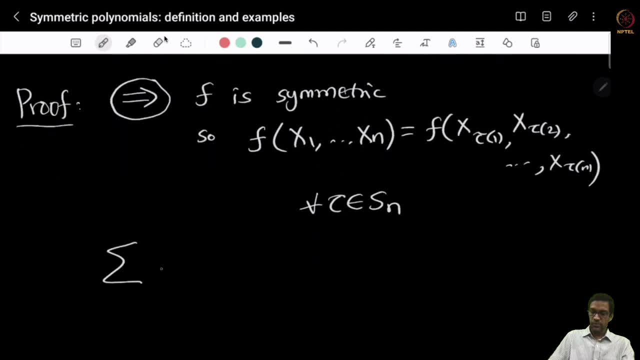 polynomial out: c, alpha x to the alpha, that is, the left hand side, f of x 1, x 2,, x n, whereas what is the right hand side? that is, I have to permute my variables. So what does that mean? I keep. 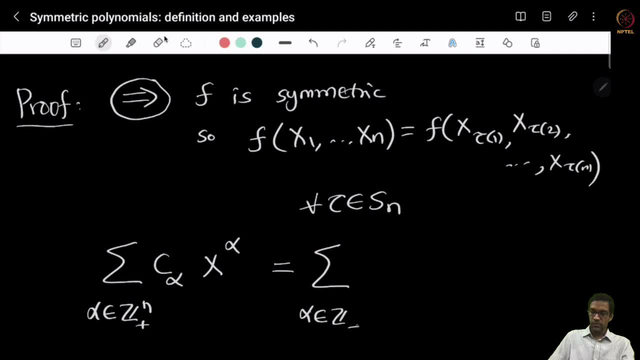 z plus n, c, alpha. and now remember what is x to the alpha. So let us write that out. what is x to the alpha? this guy is just x1 to the alpha1,, x2 to the alpha2, and so on. Now I should permute my variables. So what do I do? instead of x1, I write x, tau 1. 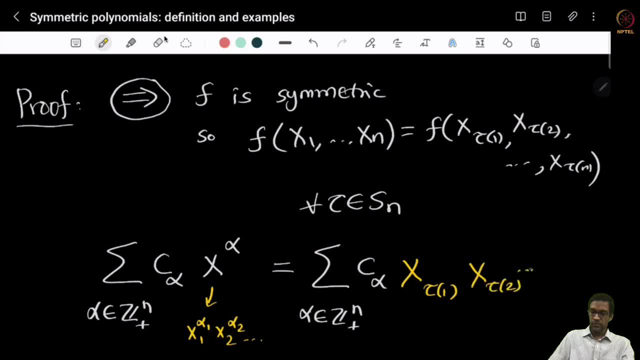 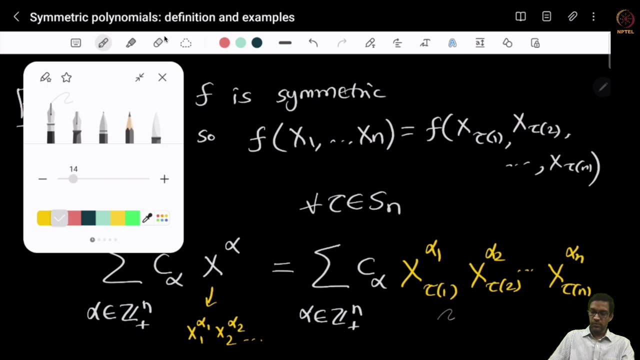 instead x2, I write x, tau 2, x tau n, but I keep my powers fixed. it is alpha1, alpha2, alpha. that is what it means: to expand and permute the variables. ok, good, so that is an equality. but now we know the following: that the coefficients, so let us compare the same. 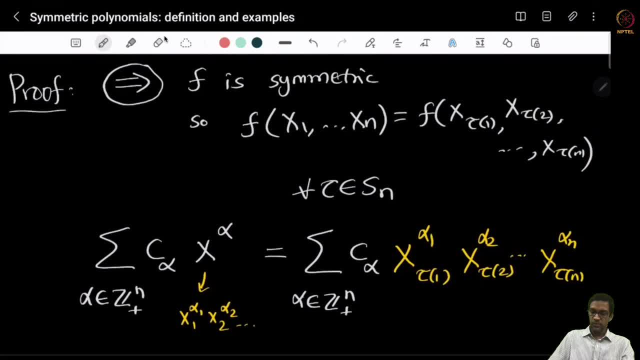 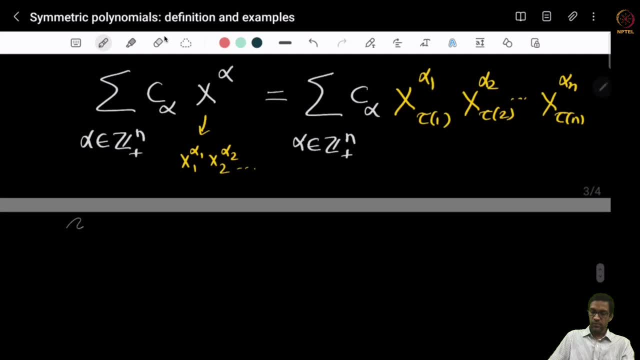 coefficient on both sides. so I am going to compare the coefficient of x power alpha on both sides of this equation. so let us do that. so compare coefficients of x to the alpha on both sides. ok, maybe we should let us choose a different. instead of alpha, let us choose. 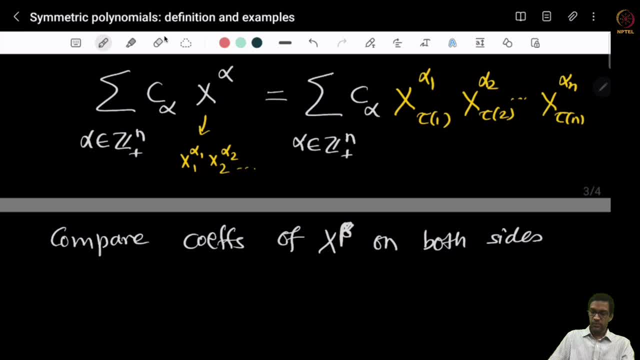 a beta here and I ask: ok, what is the coefficient of x to the beta on both sides of this equation? on the left hand side, it is easy with the coefficient of the monomial x to the beta to the beta is just c beta on the left hand side. Now, what is it on the right hand side? that is? 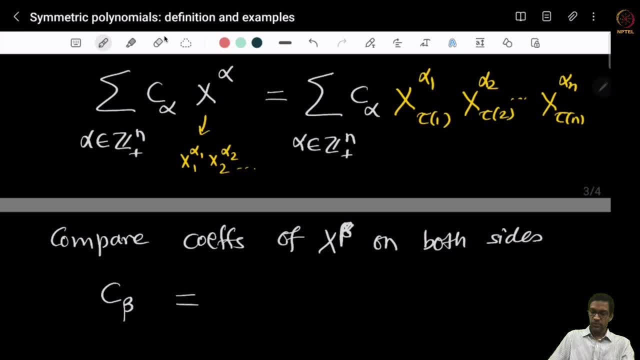 really the question. Now, on the right hand side, I need to pick out the monomial x 1 to the beta 1, x 2 to the beta 2, and so on. Now, when will I get that monomial? for which alpha in this? 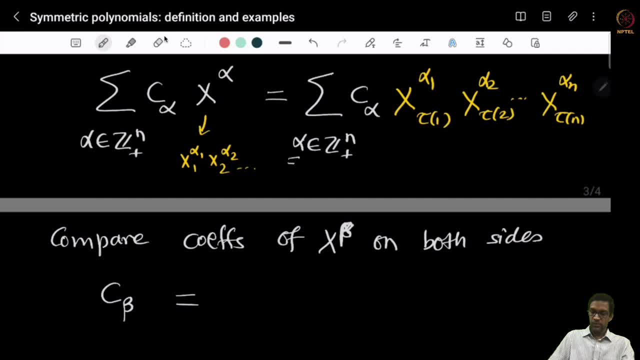 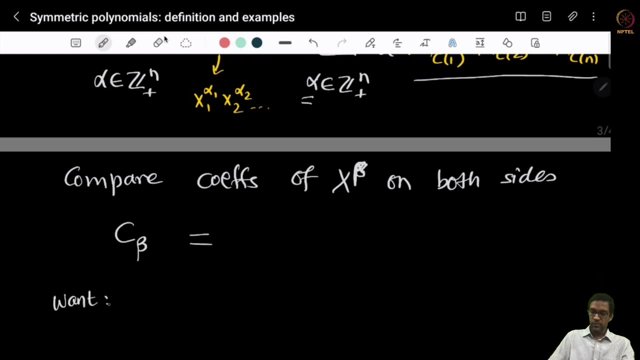 summation: will I, will this monomial become the monomial x to the beta? So let us ask ourselves that question. So when will this become x to the beta? let us do it on the side. So what I want is: well, I have this monomial here, So x to the tau 1.. 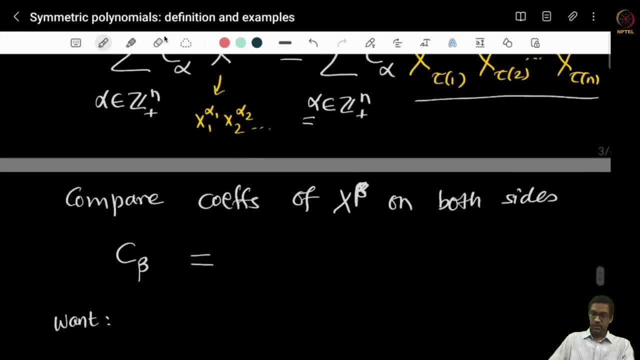 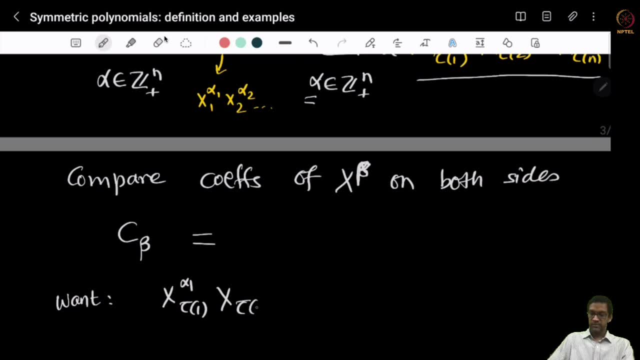 So I want this: x tau 1 to the alpha 1, x tau 2 to the alpha 2, and so on. tau n to the alpha n. I want this monomial to be the monomial x to the beta, which means it is x 1 to the beta 1, x 2 to the beta 2 is. 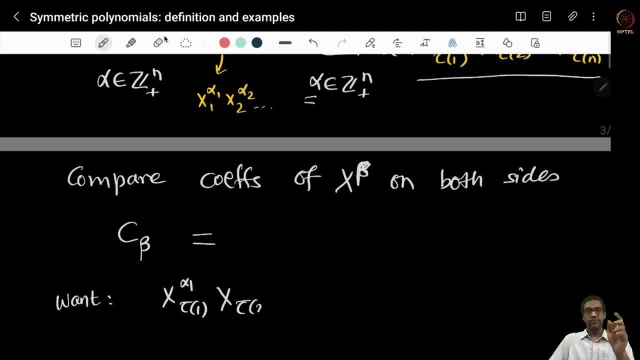 So this is sort of the observation we made: either you keep the powers in place and you permute the variables, or that same term you can think of as being obtained by keeping the variables fixed and permuting the powers. So that is what is going to happen now. 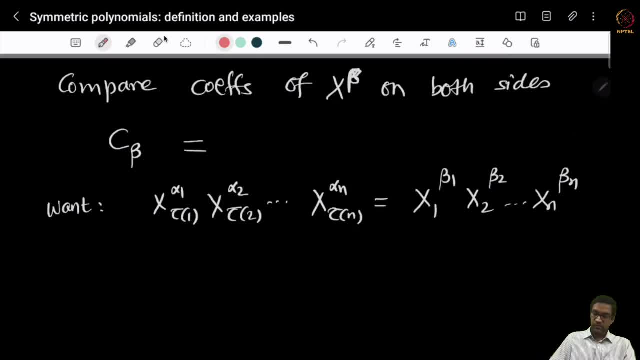 So let us compare both these sides. Now I want to compare these two. I know that they are the same, So what does it mean? So let us see, among these guys here, these subscripts 1 will occur somewhere, So there will be some term for which this tau of that is 1.. 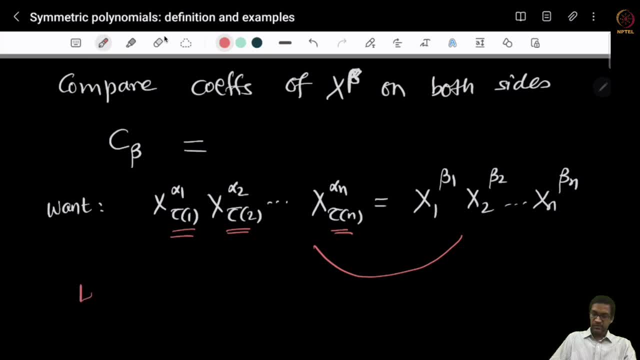 So look at, so let us call it something. let k be such that tau k is 1.. Then what does it mean? It means that what is the power I will get here. So on the left hand side it will look like this: I have a bunch of terms and then I have x, k. 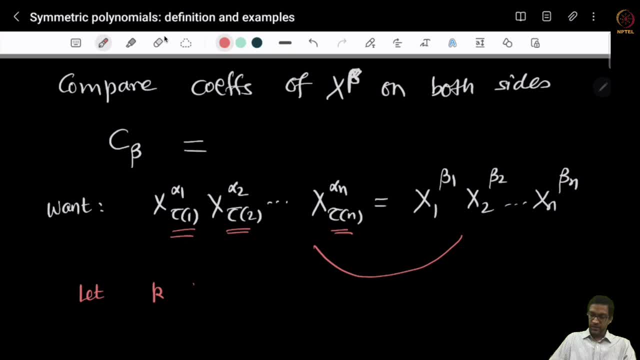 power. sorry, x, tau k, x, tau k. power, alpha k and tau k is just the number 1 here. So this is just going to look like dot dot dot. So these are the other earlier terms, and then this is x 1.. So this is just going to look like dot dot dot. So these are the other earlier terms, and then this is x 1.. 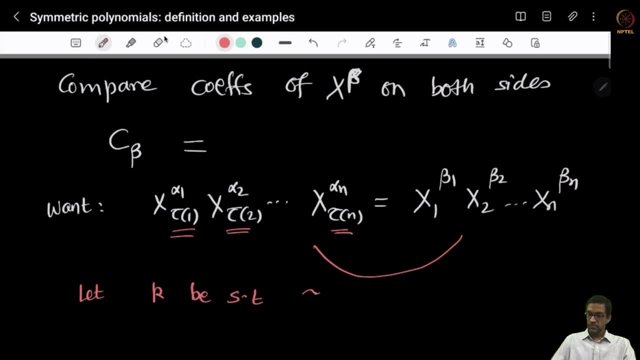 So I know that these two have to be equal to each other. this term and this term are equal. What does that mean? It means that alpha k has to be the number beta 1.. So that just tells me beta 1. 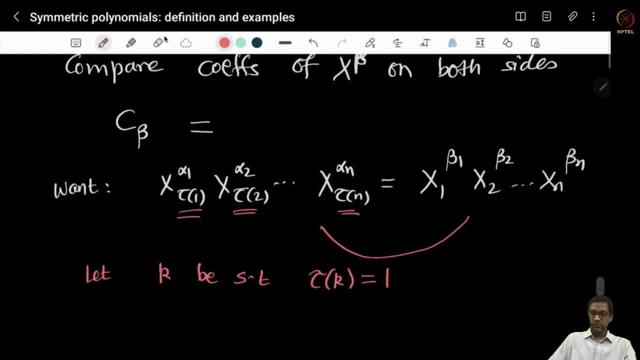 had better equal the number alpha k. But what is alpha k? What was k really? k is a number such that tau k is 1.. So this is just alpha of tau inverse of 1.. k is just tau inverse 1.. 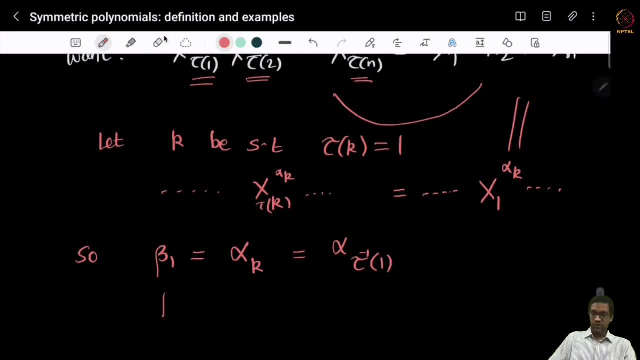 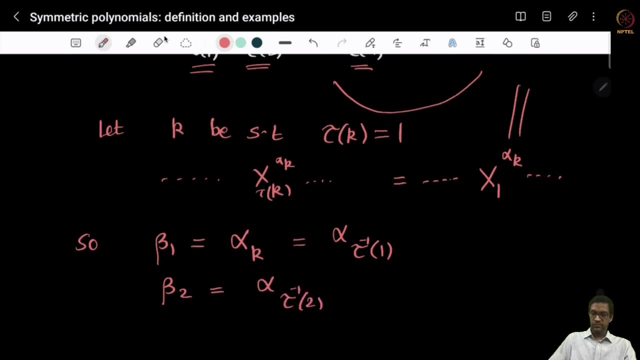 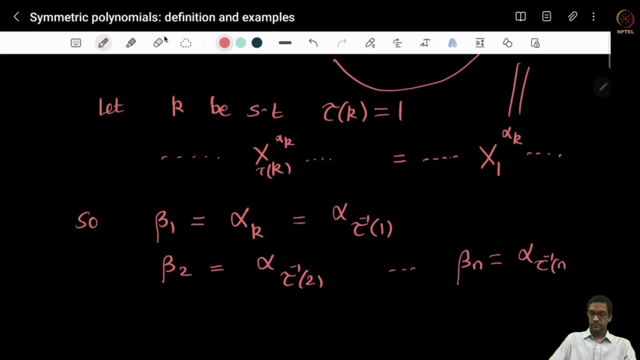 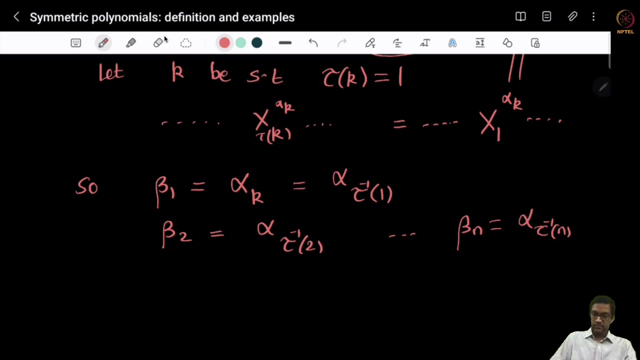 Now, similarly, you just continue with the same argument. you will conclude that beta 2 has to coincide with alpha of tau, inverse 2, and so on all the way till beta n, Or equivalently. one can invert this relation. Let us rewrite it as follows: equivalently: 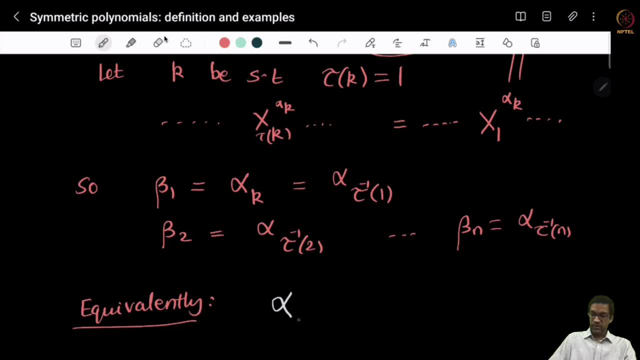 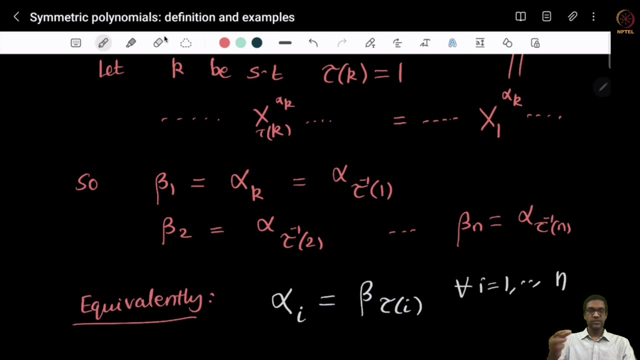 Let me write alpha. I can write it as this: alpha i is nothing but beta. tau of i For all i equals 1 to alpha. It is the same thing. I have just rewritten it now in terms of tau in rather than tau inverse Good. 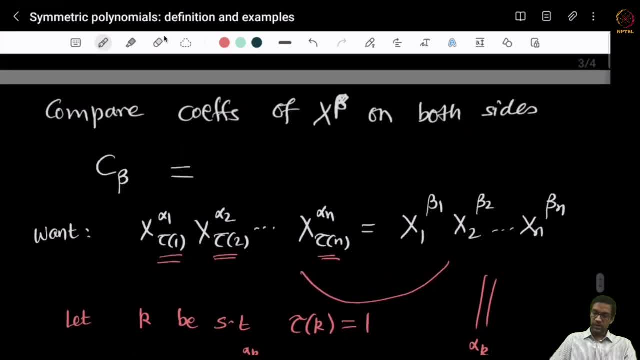 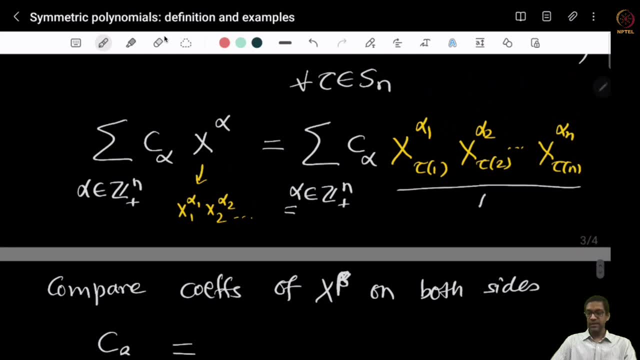 So what does that mean? Let us go back up. So we figured out. if I want to get this term to be the term x to the beta on the left side, then the alphas have to just be tau of the betas. 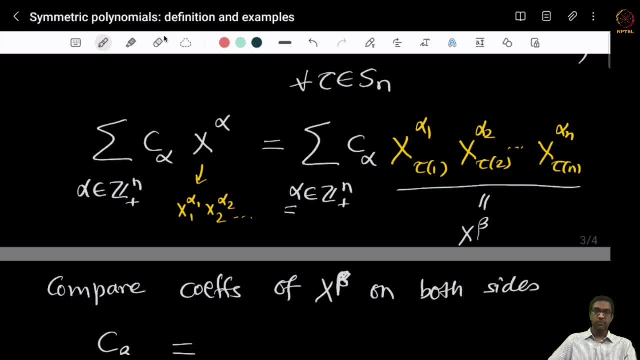 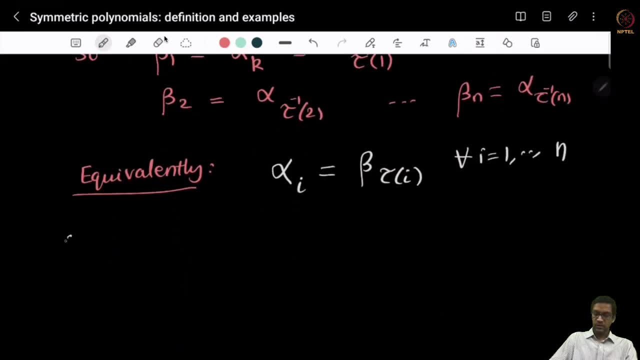 So the coefficient that I am going to get is just c sub tau of the betas. so therefore coefficient. therefore, we conclude that the coefficient of the term X to the beta on the right-hand side of this equation is nothing but C sub the alphas. where alphas are these guys? beta tau, i's, beta tau 1, beta tau 2. 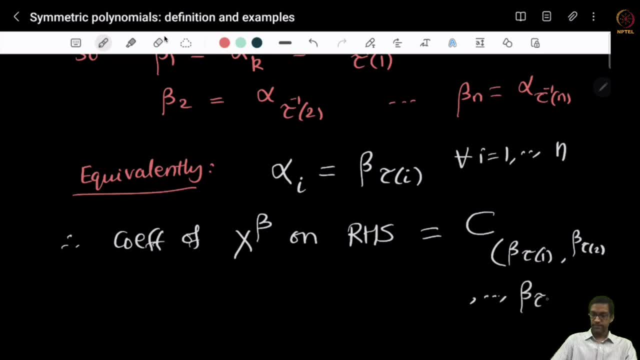 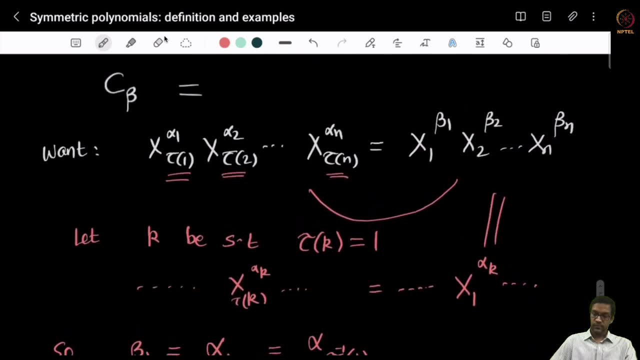 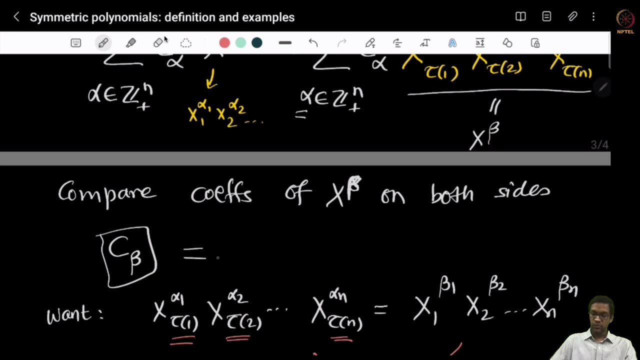 okay, and let's go back up. we already knew what the coefficient was on the left-hand side. that was C beta. okay, so should upset the coefficient of the left-hand side, is this okay? so now the equality coefficients on left and right side are equal. therefore, we conclude that.